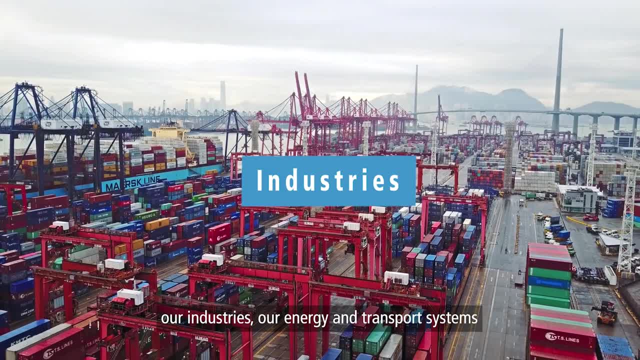 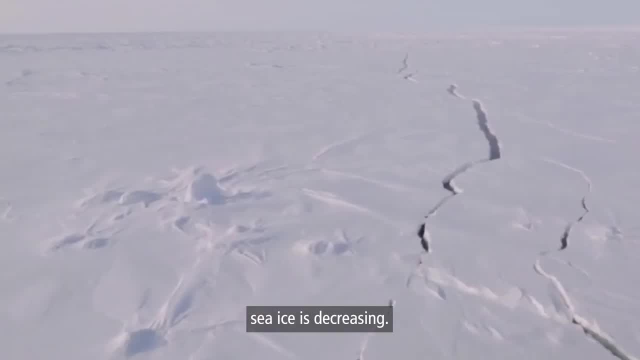 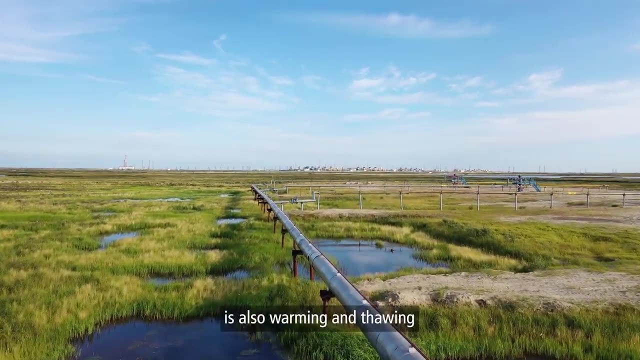 our culture and identity, our industries, our energy and transport systems, our cities and infrastructure. In our Arctic region. sea ice is decreasing. Ground that has been frozen for thousands of years, called permafrost, is also warming and thawing, causing buildings and infrastructure. 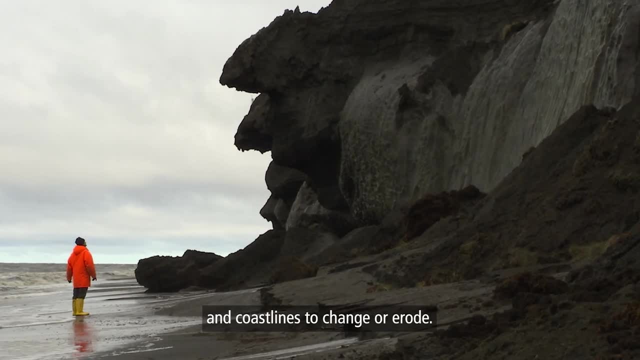 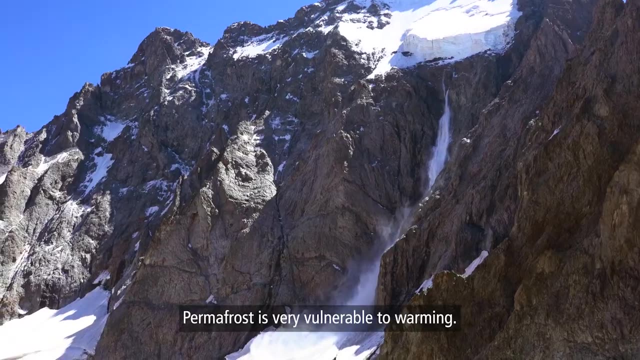 to collapse And coastlines to change or erode. Widespread permafrost thaw is expected by the turn of the century. Permafrost is very vulnerable to warming. Also contained within this permafrost is a vast amount of carbon. 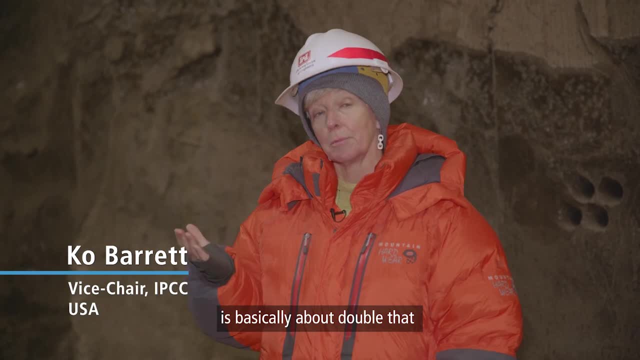 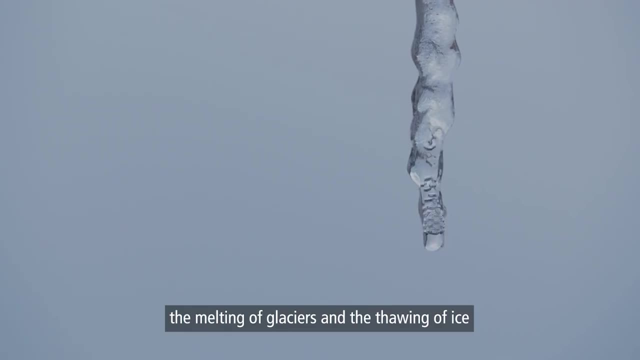 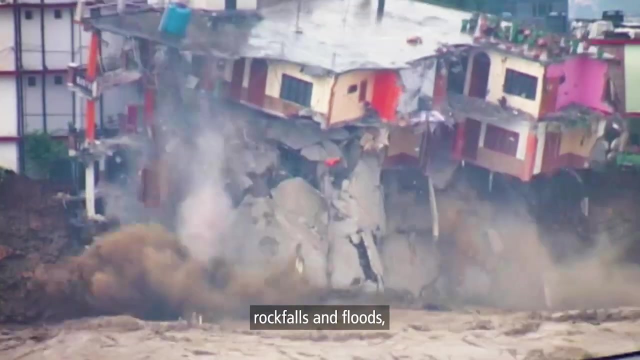 The amount of carbon that's stored in permafrost is basically about double of that contained in the atmosphere at present. In high mountain regions, the melting of glaciers and the thawing of ice and permafrost are increasing hazards such as landslides, avalanches, rockfalls and floods, while also affecting 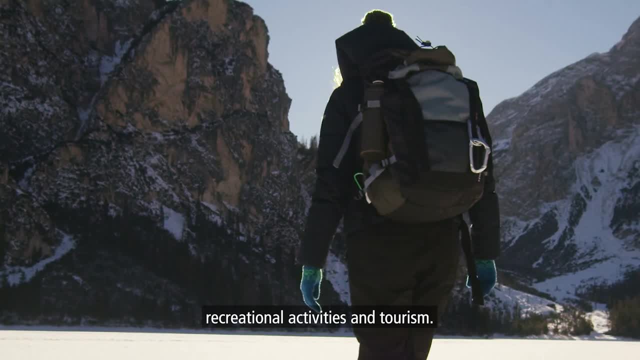 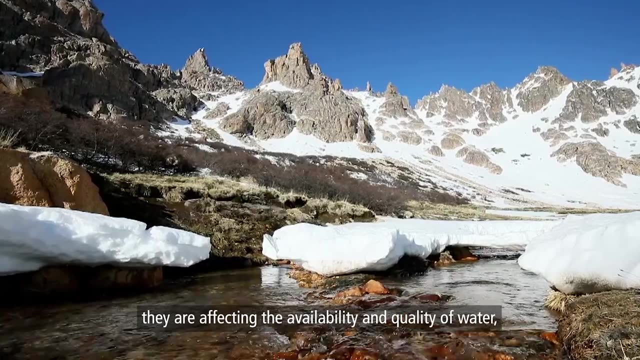 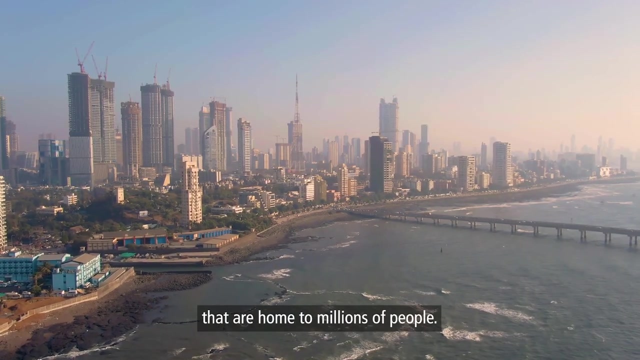 cultural heritage, recreational activities and tourism. As high mountain glaciers retreat, they are affecting the availability and quality of water Not only for high mountain communities, but for agriculture, hydropower and cities downstream that are home to millions of people. When glaciers melt, they release water. 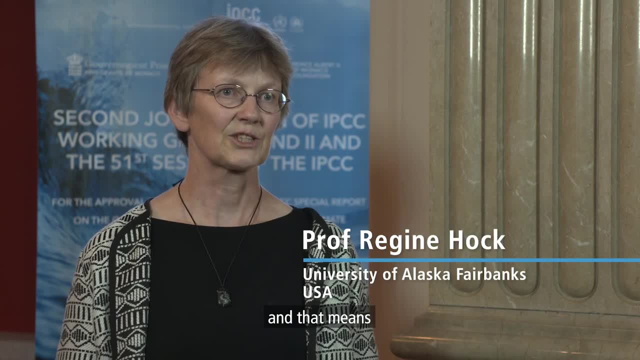 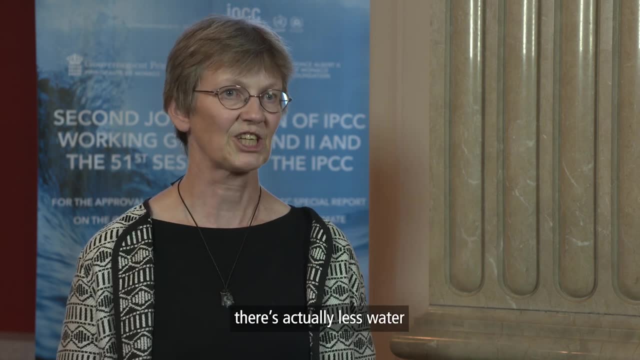 We release water that is stored in the glacier, and that means first, when the melt occurs, there's more water because of the melt, but as the glaciers retreat and shrink, there's actually less water available for agriculture, for hydropower and so on. 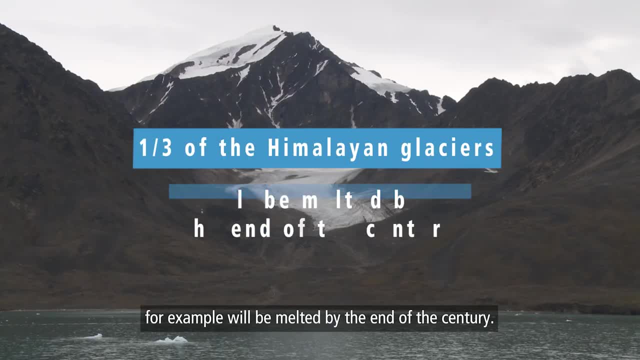 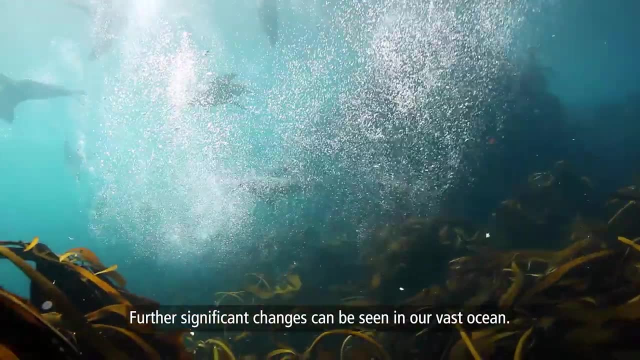 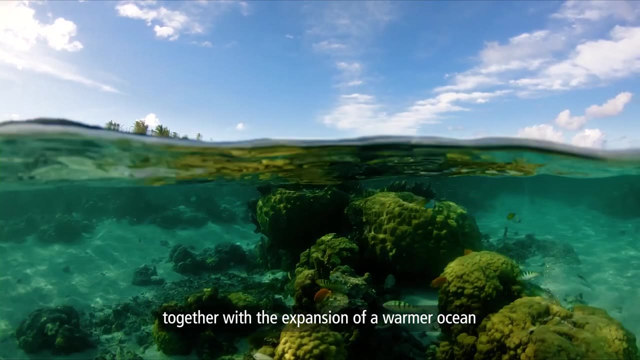 About one third of the Himalayan glaciers, for example, will be melting by the end of the century. Further significant changes can be seen in our vast ocean. Rising glaciers and ice sheets, together with the expansion of a warmer ocean, are causing. 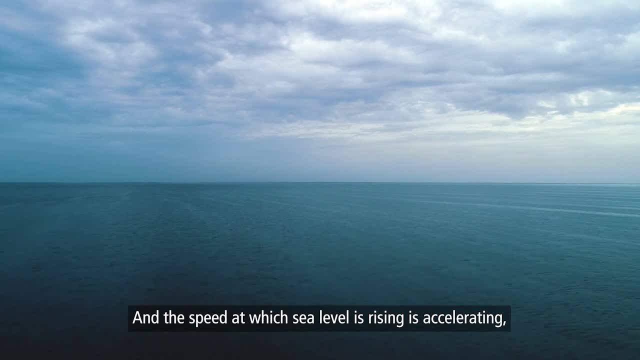 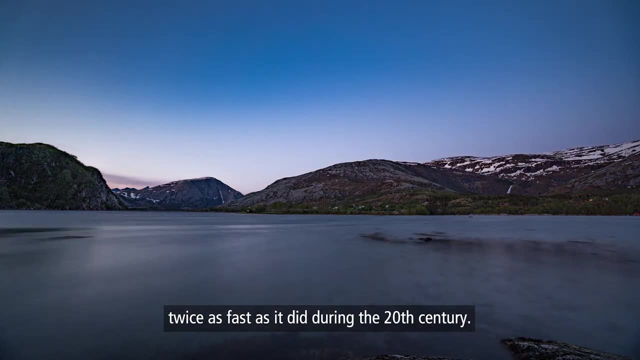 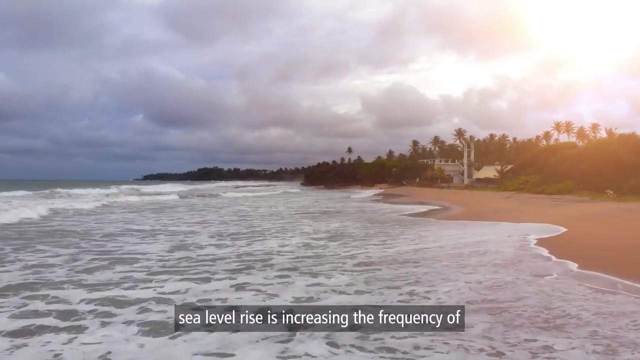 sea levels to rise, And the speed at which sea level is rising is accelerating, with our global sea level rising twice as fast as it did during the 20th century. In low-lying coastal megacities and on small islands, sea level rise is increasing the 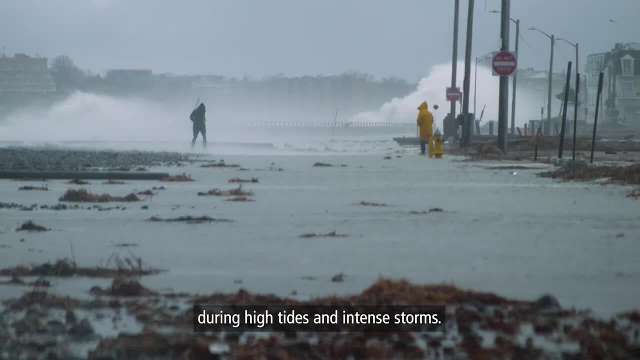 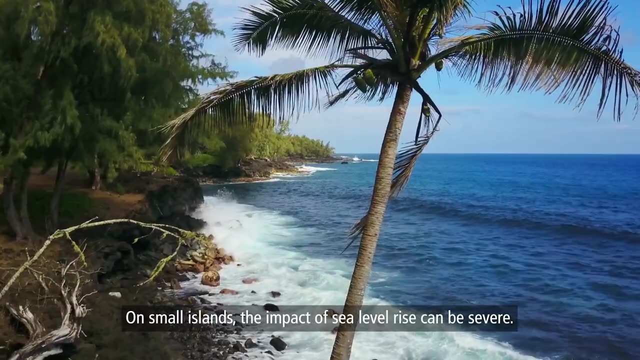 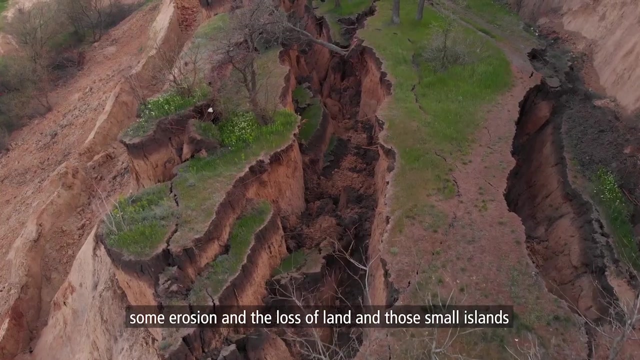 frequency of extreme sea level events. during high tides and intense storms On small islands, the impact of sea level rise can be severe. Well, you have, first of all, some erosion and the loss of land, and those small islands there do not have that much land to start with. 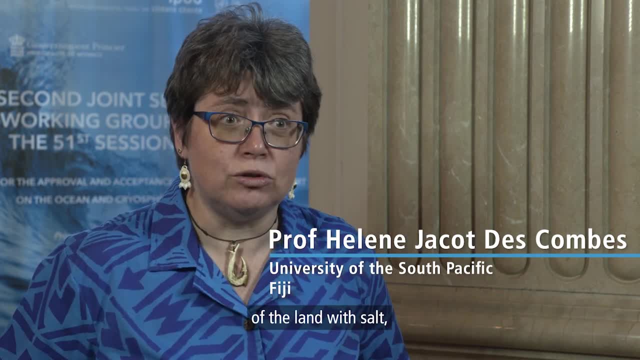 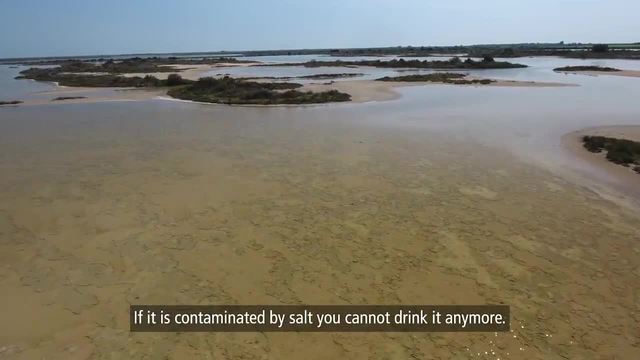 You also have the problem of the contamination of the land with salt and on the water that is stored under that land. if it is contaminated by salt, you cannot drink it anymore, And if your soil is contaminated by salt you cannot grow the crops. 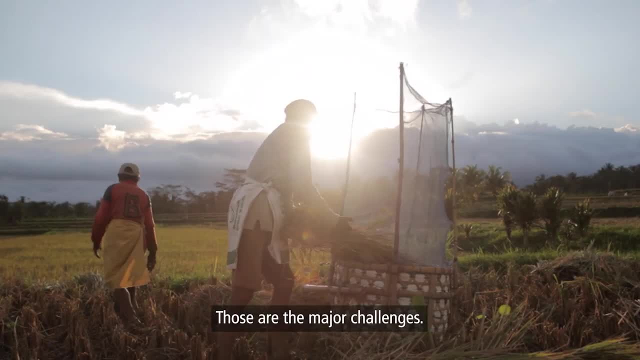 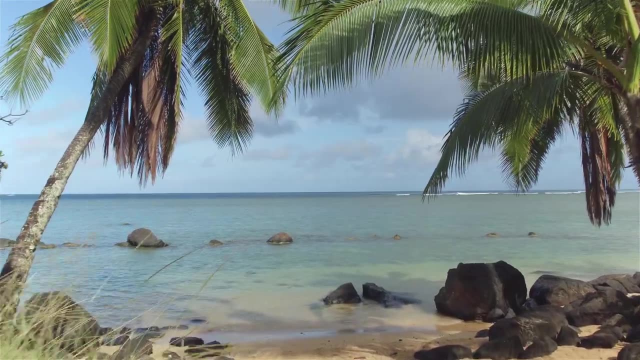 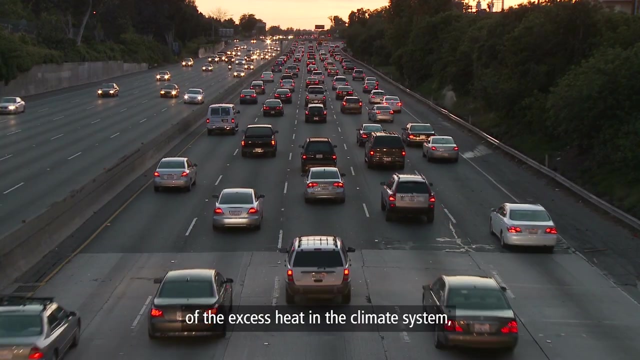 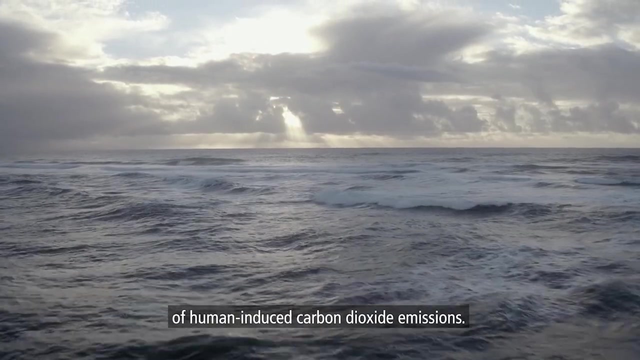 and the vegetables. So you have food supply and health issues. Those are the major challenges. Over the past few decades, our ocean has absorbed more than 90 percent of the excess heat in the climate system and taken up between 20 and 30 percent of human-induced carbon dioxide emissions. 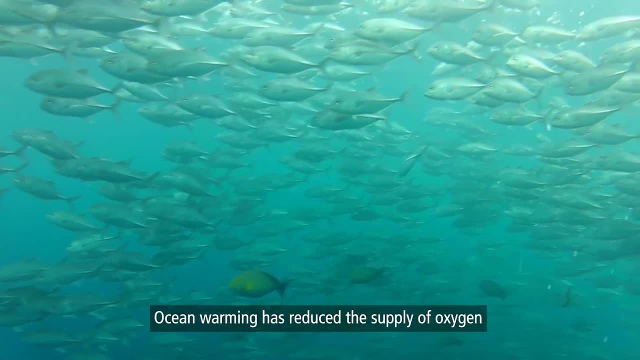 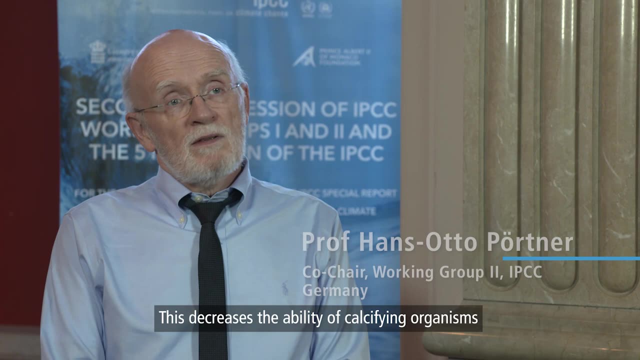 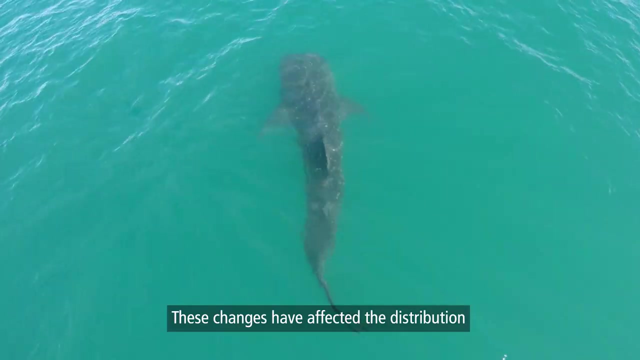 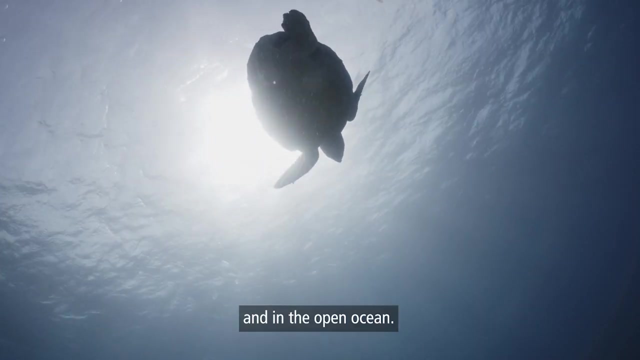 Ocean warming has reduced the supply of oxygen and nutrients to marine life, while increasing CO2 levels cause ocean acidification. This decreases the ability of calcifying organisms to build shells and skeletons. These changes have affected the distribution and abundance of marine life in coastal areas and in the open ocean Across the world. we are already starting to respond. 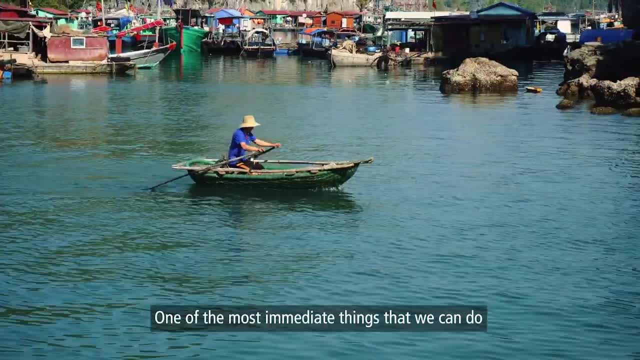 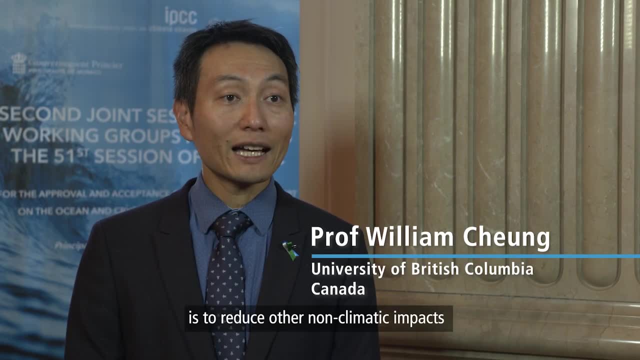 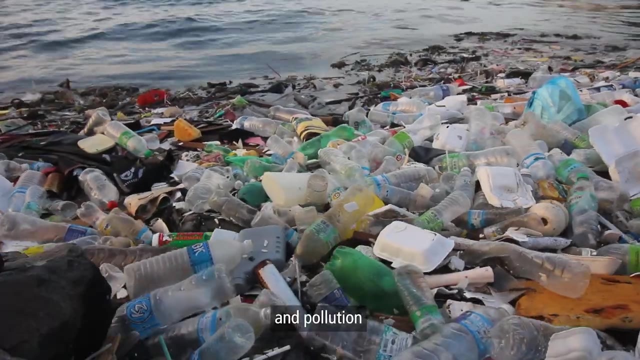 and adapt to changes in our ocean and cryosphere. One of the most immediate things that we can do is to reduce other non-climatic impacts on marine ecosystems and the oceans. Overfishing, habitat destructions, pollution can exacerbate the impacts of climate change. 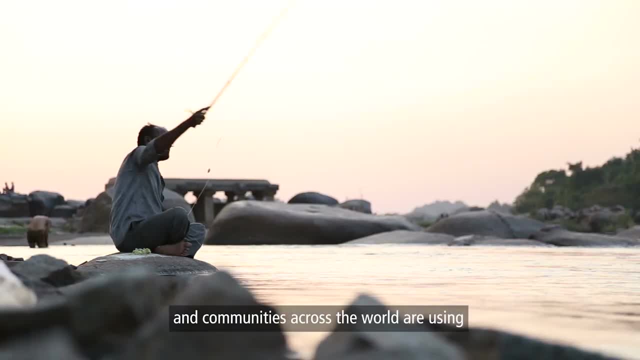 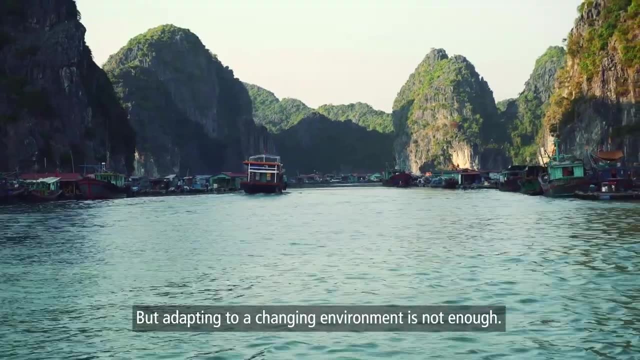 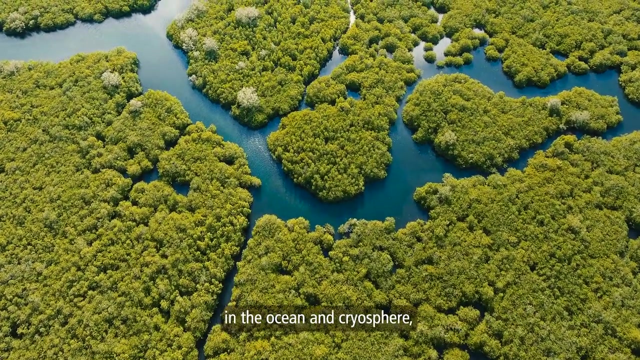 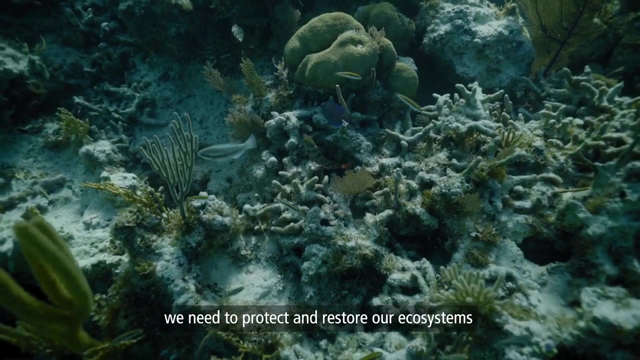 Climate change are very local, specific, and communities across the world are using their own knowledge to adapt. But adapting to a changing environment is not enough To address unprecedented and long-term changes in the ocean and cryosphere and safeguard our livelihoods and communities. we need to protect and restore our ecosystems.